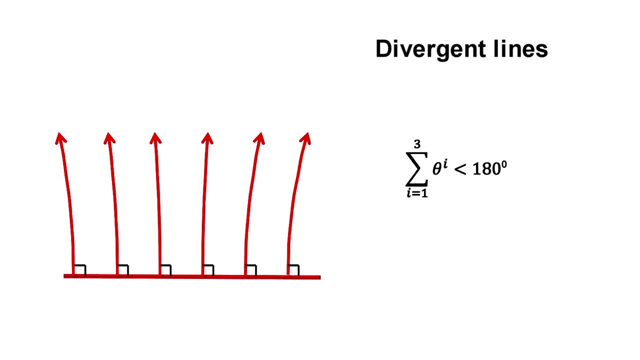 space is stretched Here. the sum of the angles of a triangle is less than 180 degrees and the circumference of a circle is more than 2 pi times its radius. This is hyperbolic geometry. It represents space with a negative curvature. The best example of this is the 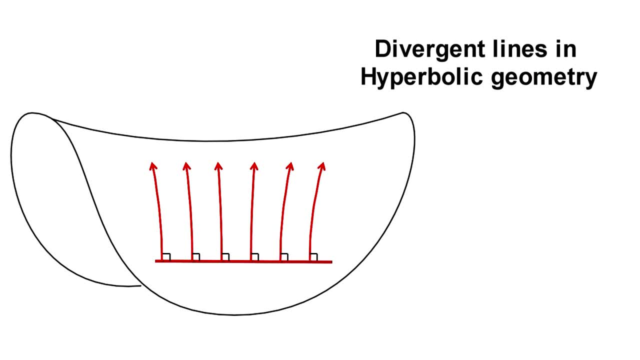 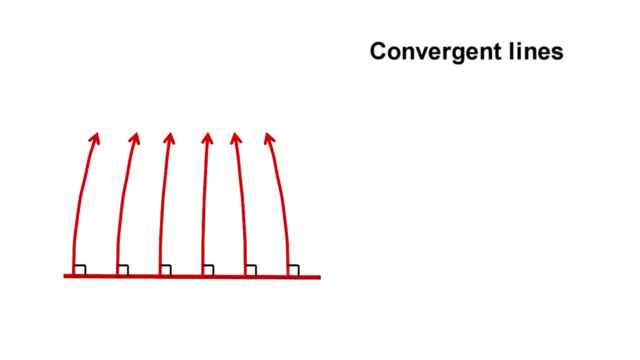 surface of a saddle or a potato chip. Another possibility for a different geometry supposes that the parallel geodesic lines are converging and will eventually meet. It's as if space were being compressed between the lines and the further up the lines you 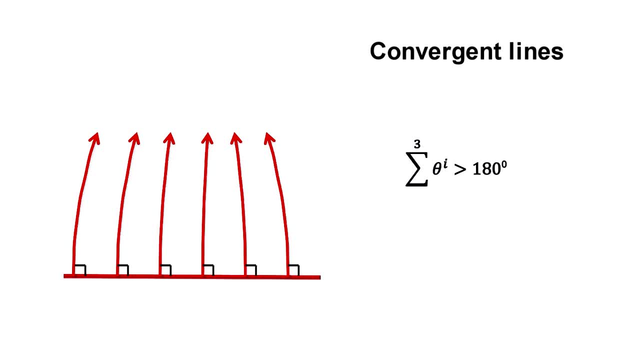 go, the more the space is compressed. Here, the sum of the angles of a triangle is greater than 180 degrees and the circumference of a circle is less than 2 pi times its radius. This is spherical geometry. It represents space with a positive curvature. The best example of this is the surface of a sphere. 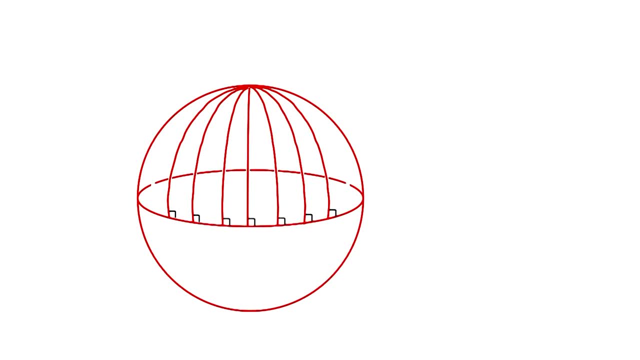 like the Earth itself. Here, the curvature is constant throughout the surface. The baseline is the equator, The perpendicular line is the depth and the curvature is the radius. This is a curve that is constant throughout the surface. The baseline is the equator. 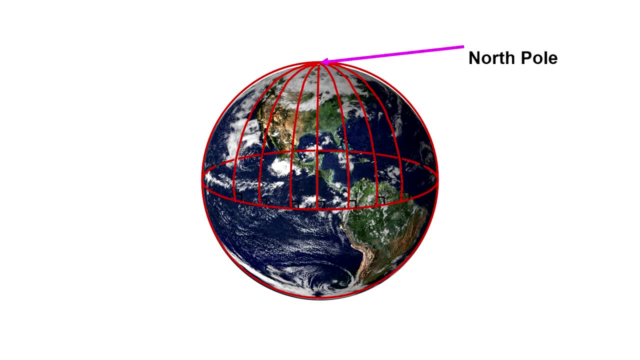 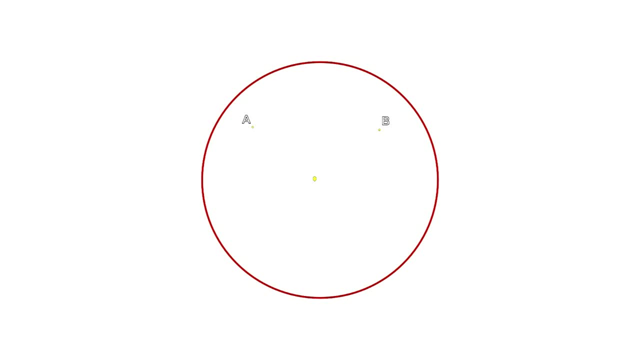 The perpendicular line is the diameter, The curvature is the depth, The curvature of the are the lines of longitude and they meet at the North Pole. Here's the best way to find the geodesic between two points on a sphere. First, intercept the sphere with a plane that contains the two points plus the center. 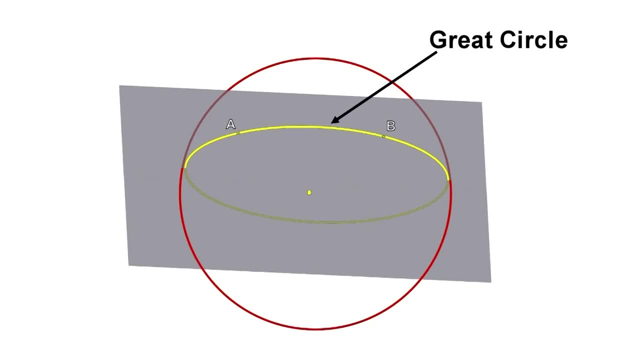 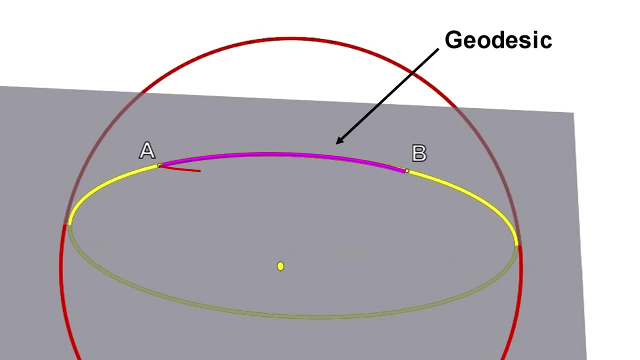 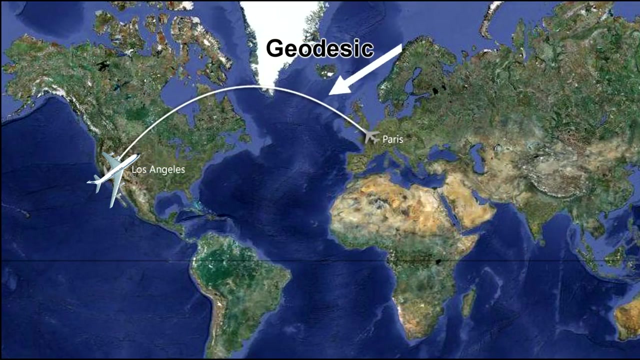 of the sphere. The intersection is called a great circle. The segment of the circle that connects the two points is the shortest distance between the two points. A parallel of latitude line between the two points would be longer. This is why planes in the Northern Hemisphere travel north and then back. 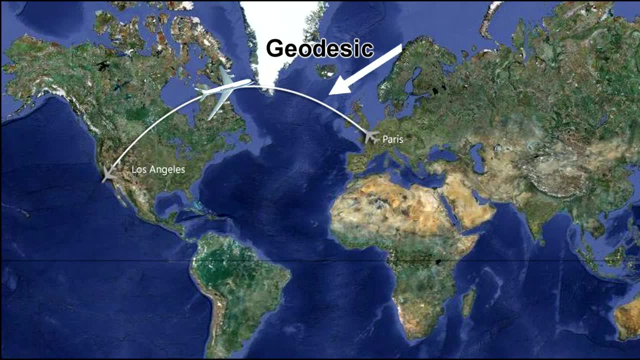 south to get to a destination at the same latitude. rather than travel due west or due east, They have chosen the shortest distance between the two points, to save on both time and fuel. Some geodesic routes can save up to a thousand kilometers. Of course, when it comes to a more generalized curved space, the curvature,